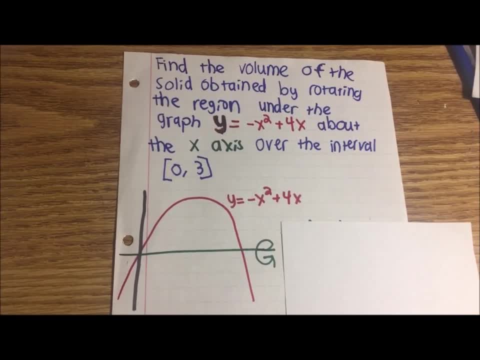 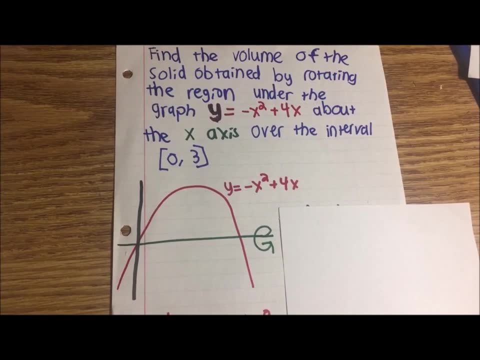 So, for example, we'll use this. Question first. The question says, find the volume of the solid obtained by rotating the region under the graph y equals negative x squared plus 4x about the x-axis over the interval 0 to 3. 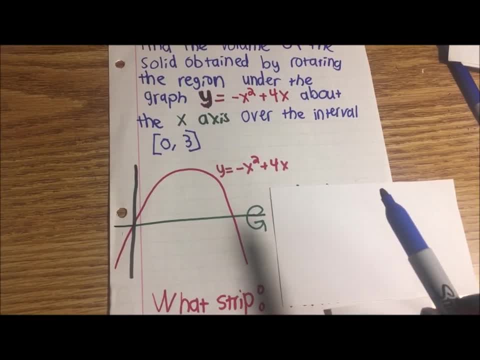 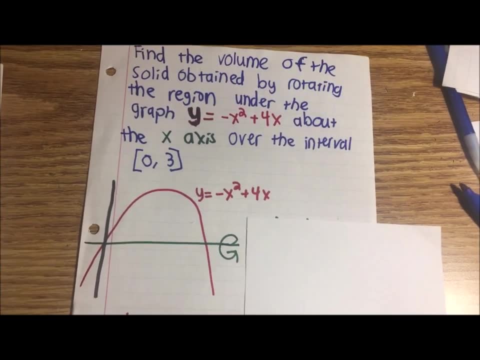 So, um, first things first, I'm guessing you guys already know how to draw a strip because of the first tutorial I did. If you guys remember this piece of paper. Um. 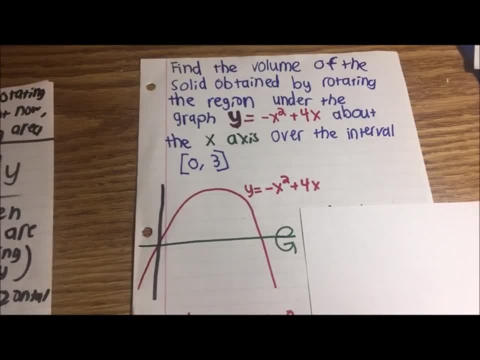 We can apply it to the same thing to figure out what's, which strip to, um, draw here. 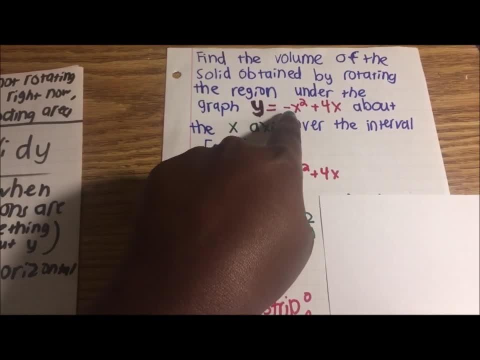 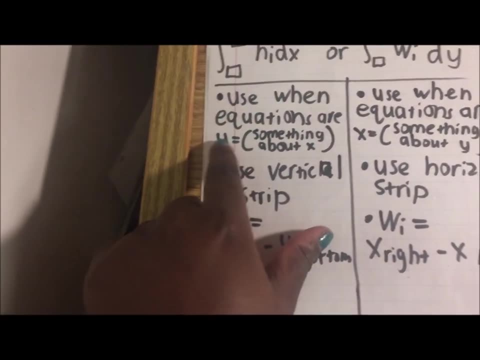 So, here it says the equation is y equals negative x squared plus 4x. y equals something about x. So, that's in this column. y equals something about x. 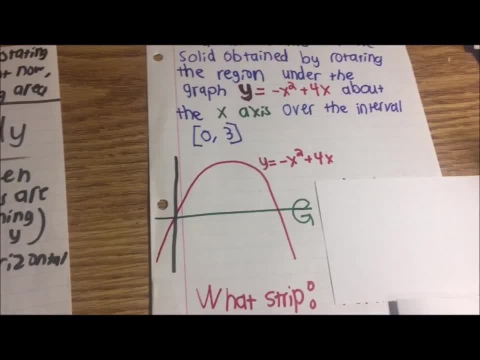 So, let's use a vertical strip. So, our strip is vertical. Let me write that. Let me draw the strip. I'll just color it in. That's our strip. Right there. There it is. Uh, yeah. That's our strip. 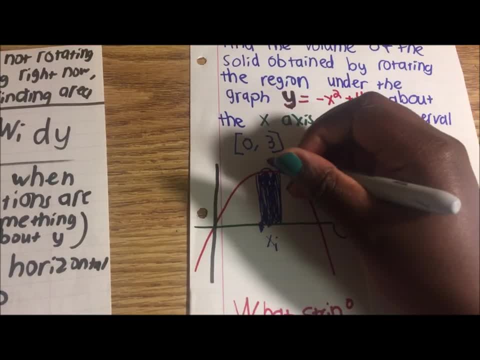 Uh, I'll just put x on here. It's good to put it there. And then dx. 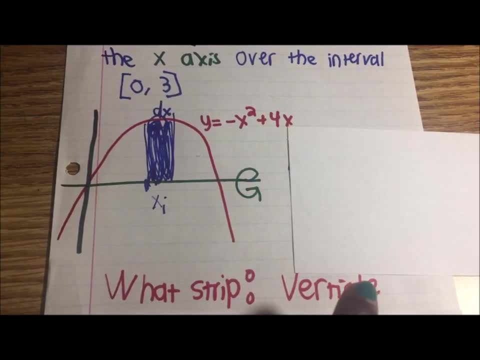 Alright, so when we asked ourselves what strip, um, we're using the vertical strip. And so, let me bring back my flowchart. 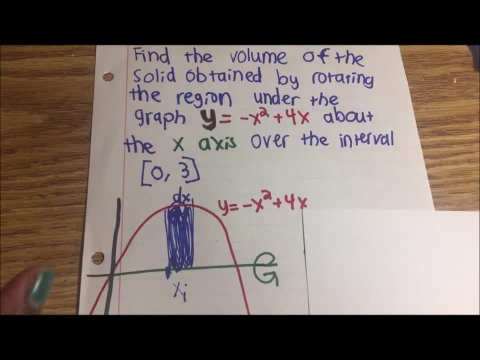 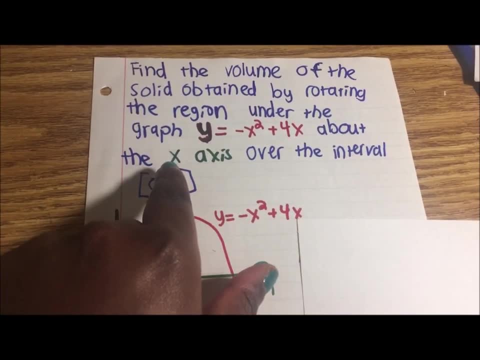 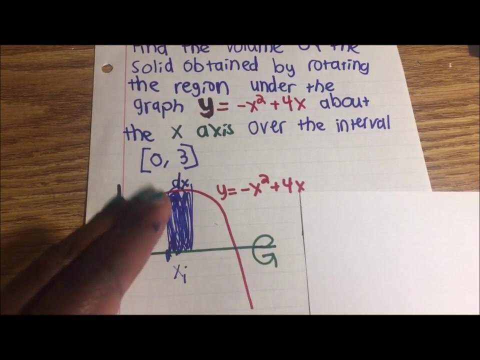 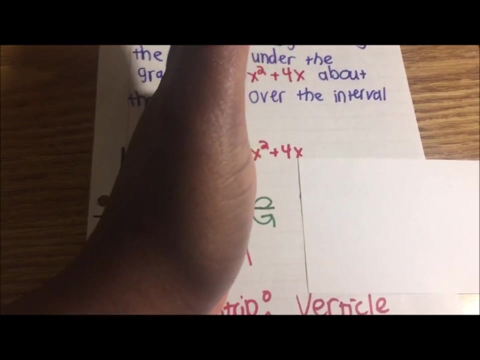 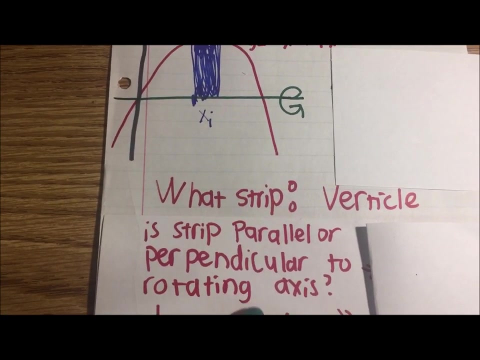 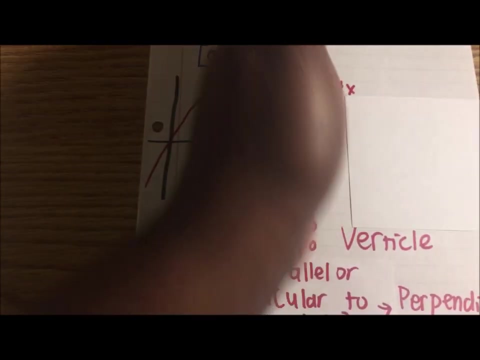 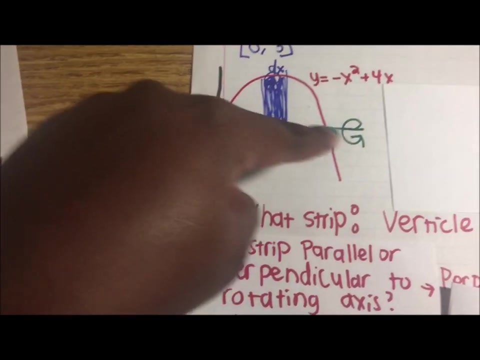 Oh, but before I do that, um, let's identify the rotating axis. The rotating axis is, they say in the, in the equation that it's being rotated about the x axis. So, I put this little like swirly thing to show that it's being rotated about the x axis. So, this is the strip, and this is the x axis. Since this is the strip, it's this way, and the rotating axis is this way, is the strip parallel, or is it perpendicular? Well, it is perpendicular! Because, the strip is like this and the rotating axis is like this. Do you guys see that? The strip is this way the rotating axis is this way. The rotating axis is the x-axis. 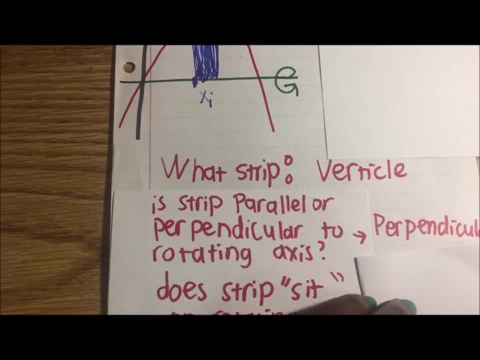 So, is the strip parallel or is it perpendicular? 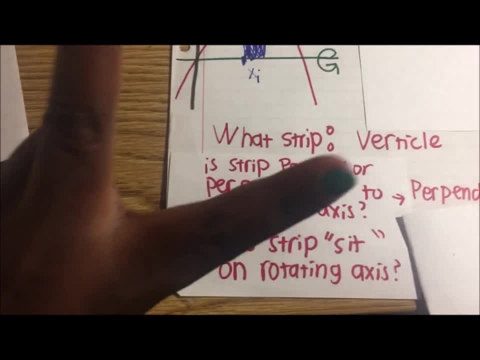 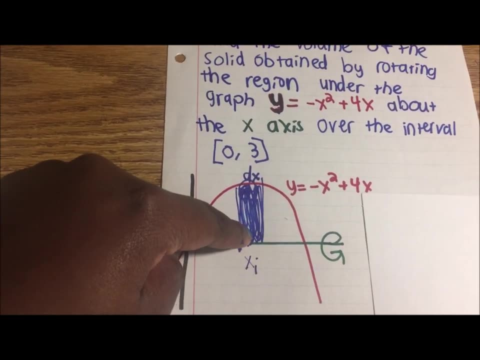 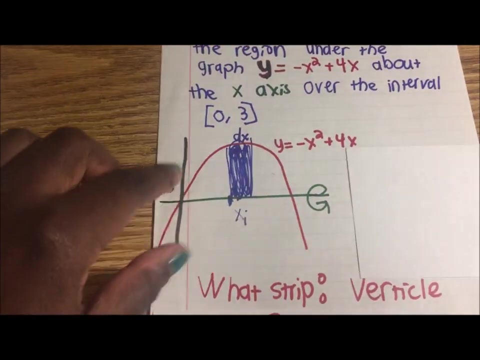 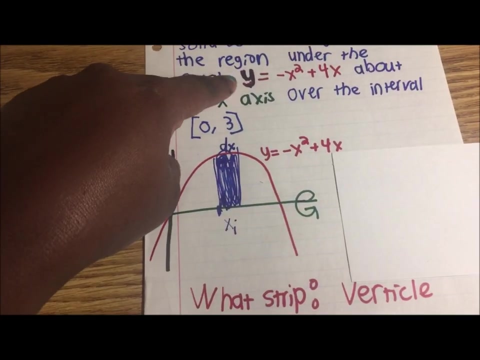 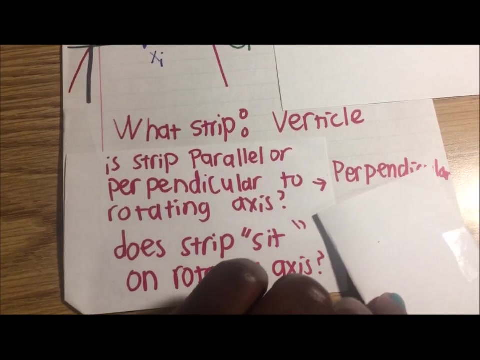 It's perpendicular. So, does the strip quote sit unquote on the rotating axis? So this is really important to know. The strip right here, it does. It sits on it. It sits right there. This strip touches the rotating axis and it sits on it. See how the strip, the bottom of the strip, it literally just touches the rotating axis? The rotating axis here is the x-axis. That's the rotating axis and the strip sits on it. So, the strip sits on the rotating axis. So, it says, does the strip sit on the rotating axis? Yes, it does. So, let's go back to our flow chart. 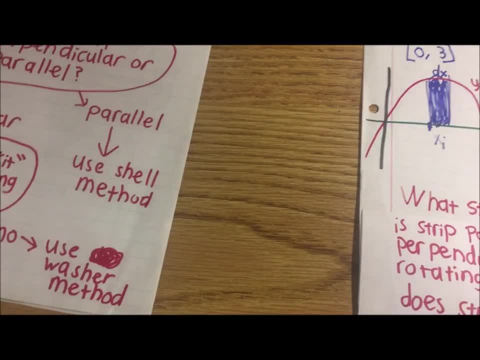 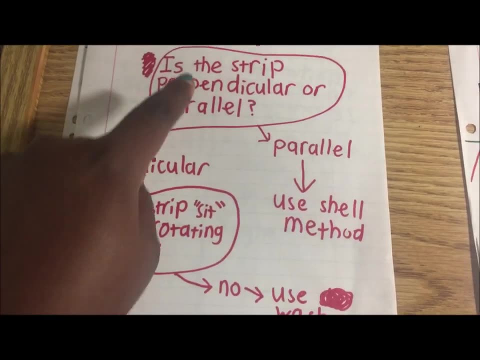 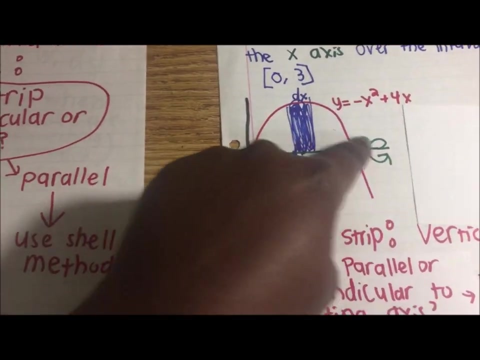 Um, let's go back to our flow chart. Is the strip perpendicular or is it parallel? It's perpendicular. So, let's go here. Does the strip sit on the rotating axis? We said yes because the strip literally just sits there on the rotating axis. So, yes. So, that means we will be using 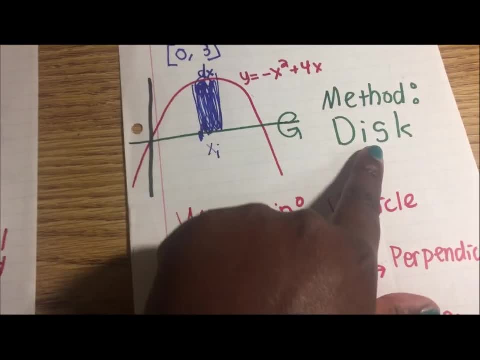 the disk method. Method to use, disk method. Alrighty, here's another example. 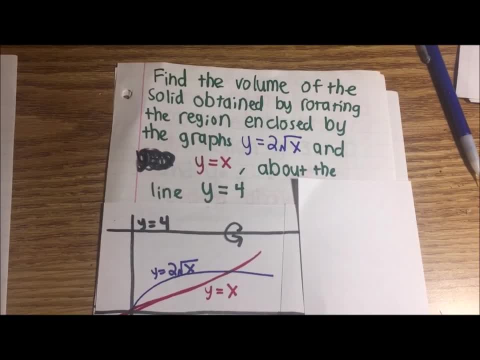 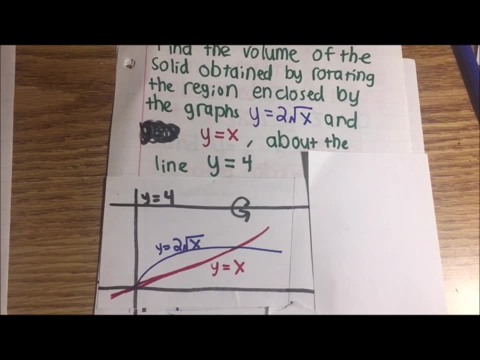 Here's another question. Find the volume of the solid obtained by rotating the region enclosed by the graphs y equals 2 times the square root of x and y equals the square root of x about the line y equals 4. 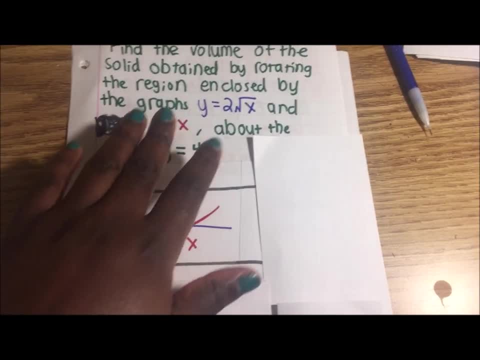 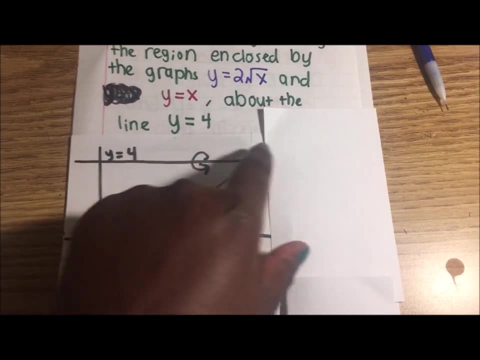 So, y equals 4 is our rotating axis. That's nothing, that's not an equation. y equals 4 is just a rotating axis because it said about the line y equals 4. So, this is our rotating axis. That's why I put the swirly thing to show that it's the rotating axis. 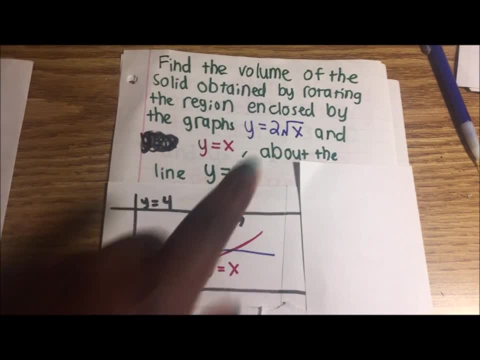 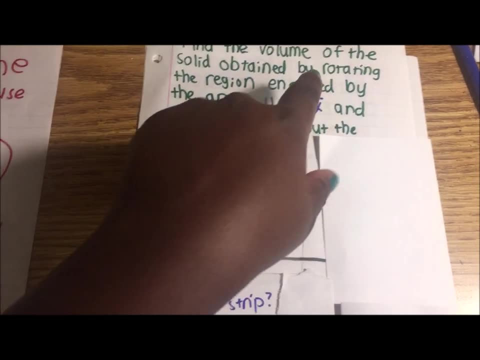 Um, the equations are y equals 2 square root of x. Square root of x and then y equals x. This right here is y equals 2 square root of x in the blue. This is y equals x in the red. So, 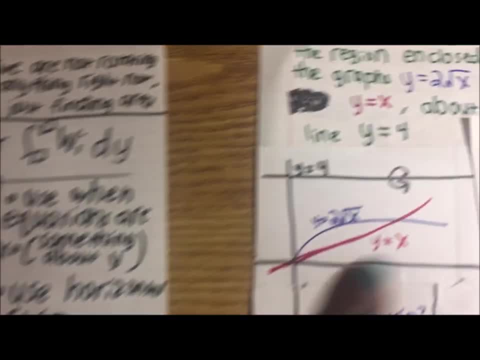 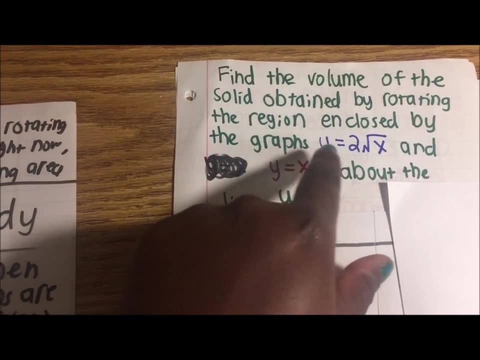 if we go back to this original paper, as you can see, the equations are y equals um, something about x, y equals something about x. 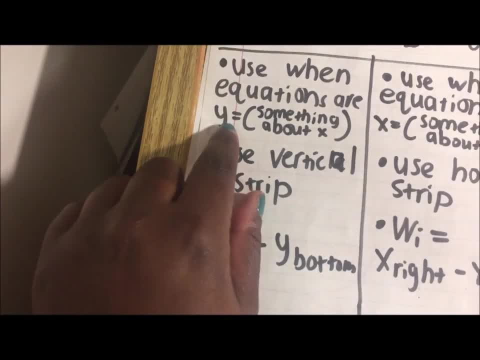 It's y equals something. So, y equals something about x. That means we use a vertical strip. 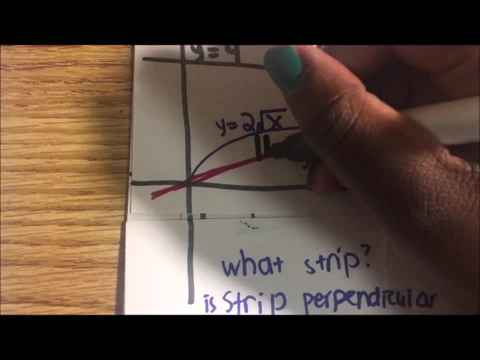 Um, the strip's kind of small. Sorry about that. But I should have drawn it bigger. But it is vertical. This is the vertical strip. 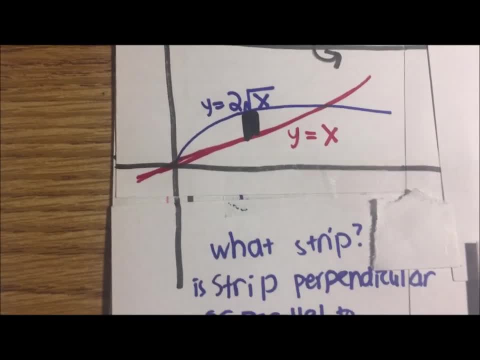 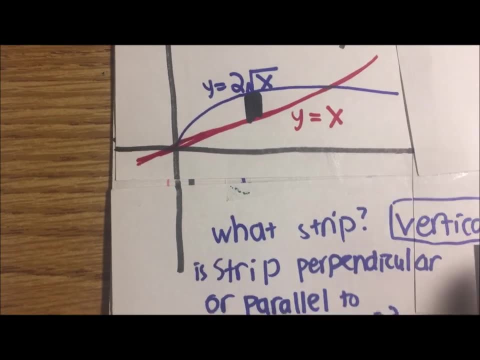 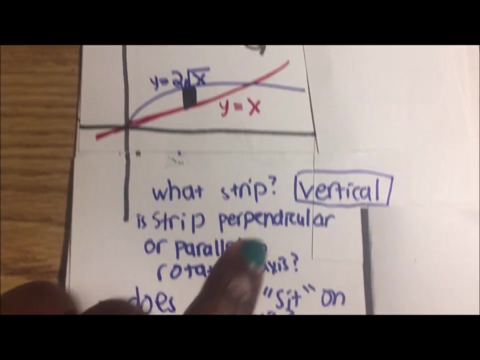 So, now let's start figuring it out. So, when we asked ourselves what strip, the strip is vertical. The strip is vertical. Now, is the strip perpendicular or parallel to the rotating axis? So, this is the strip. We said it was vertical. 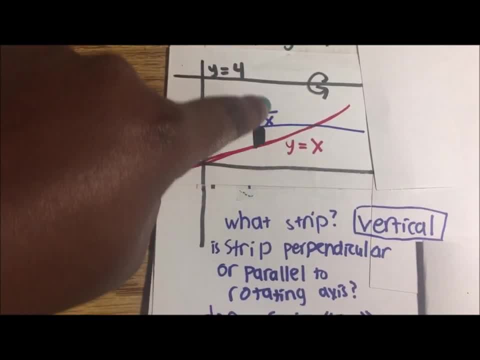 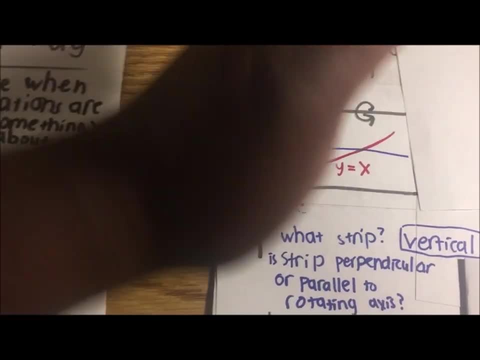 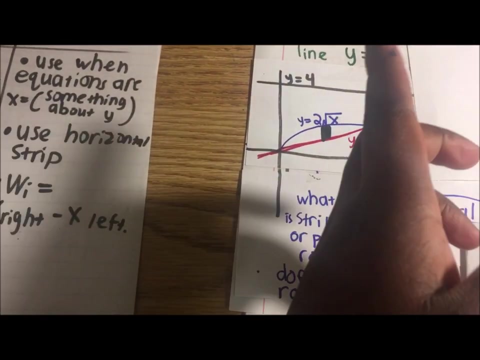 The strip is going like this. And then this is the rotating axis, y equals 4. So, y equals 4 is like this. The strip is vertical. It's like this. So, this is the rotating axis. It's like this. This is, the vertical strip is like this. 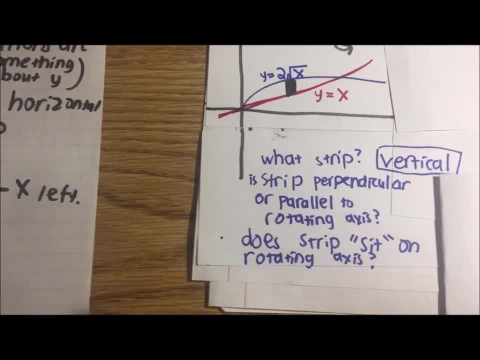 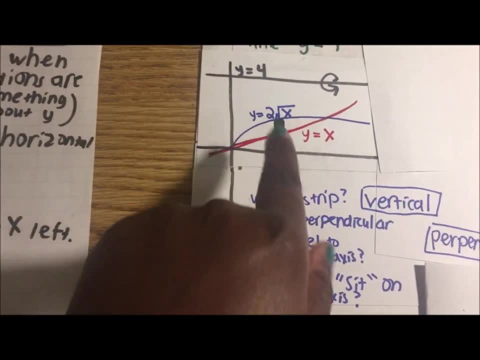 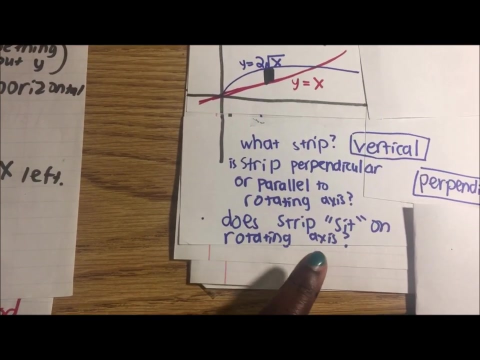 So, is the strip perpendicular or parallel to the rotating axis? It is perpendicular because this strip's is perpendicular to this, to the rotating axis. Does the strip sit on the rotating 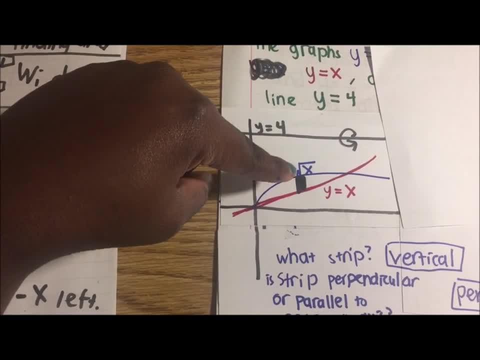 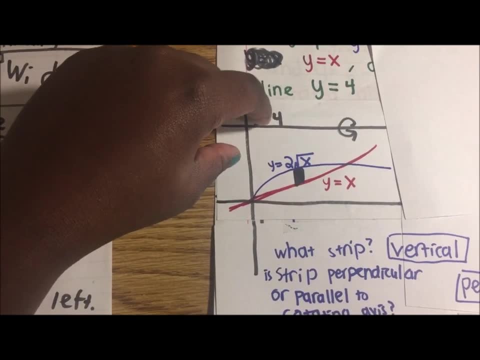 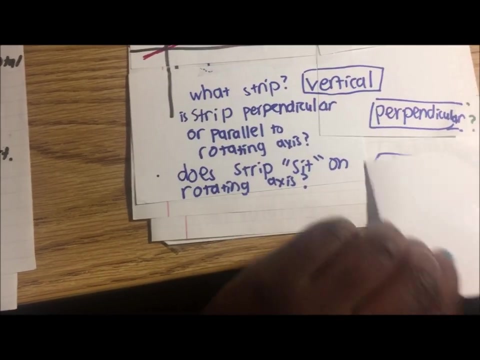 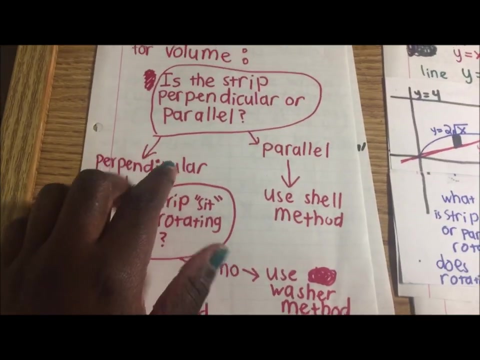 axis? Yes or no? In this scenario, no it does not because the strip is all the way down here. The strip does not touch the rotating axis. The strip does not sit on the rotating axis. It doesn't sit on it. So to answer this question, does the strip sit on the rotating axis? Absolutely not. No, it doesn't. So let's go back to our flowchart. So back to the flowchart for this one. So is the strip perpendicular or is it parallel? We said it was perpendicular because the strip 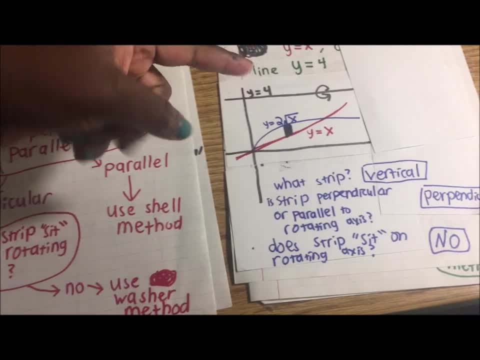 is like this and then the rotating axis is like this. So the strip is perpendicular to the rotating axis. Is it perpendicular or parallel to the 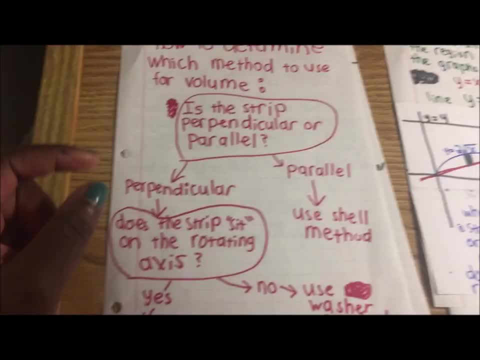 rotating axis? It is perpendicular. So does the strip sit on the rotating axis? No. It doesn't. 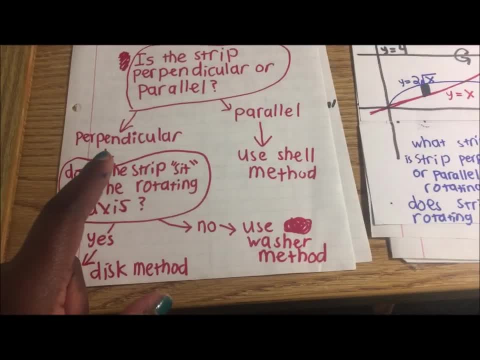 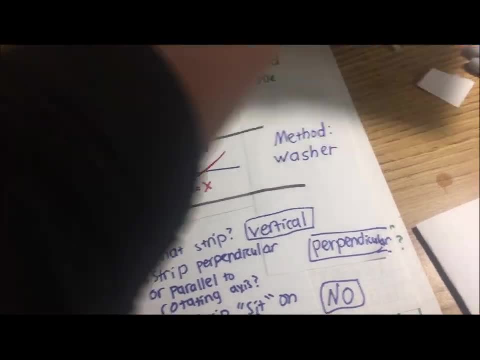 We said that it doesn't. So we said no. So that means we're going to use the washer method. The method that we use is washer. Alright, here's the third and 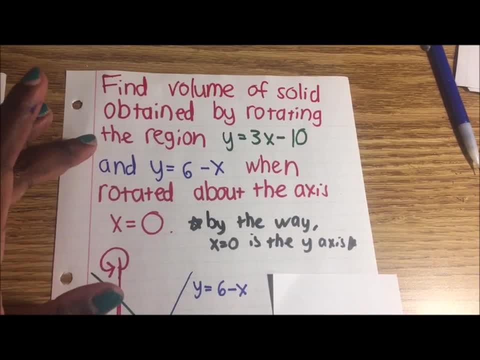 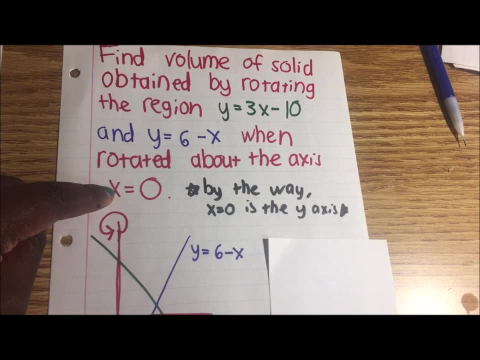 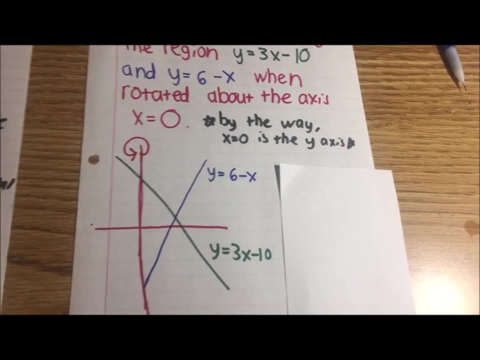 final example. Find the volume of the solid obtained by rotating the region y equals 3x plus 10 and y equals 6 minus x. When rotated about the axis, x equals 0. x equals 0 is here. So I just put, by the way, say x equals 0 is the y-axis because you know x equals 0 is the y-axis, y equals 0 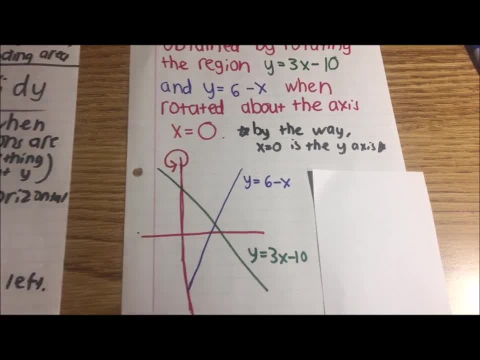 is the x-axis and so on and so forth. x equals 0 is the y-axis. So this is the region. 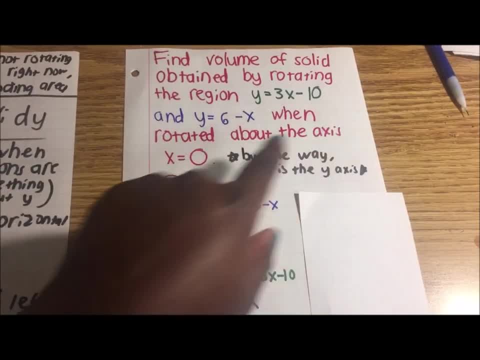 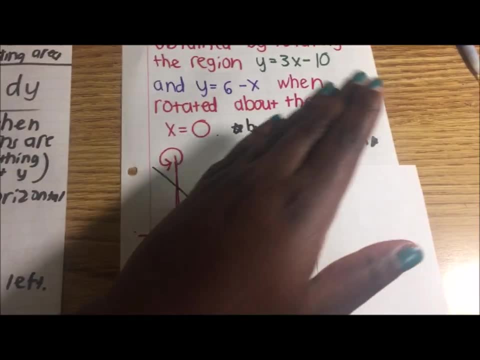 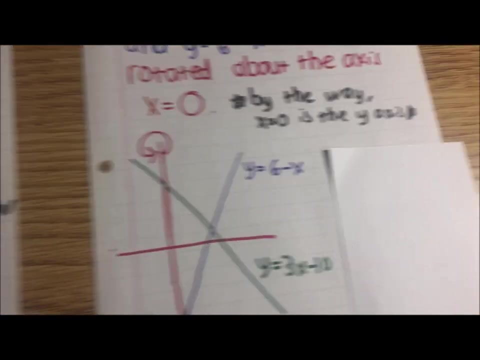 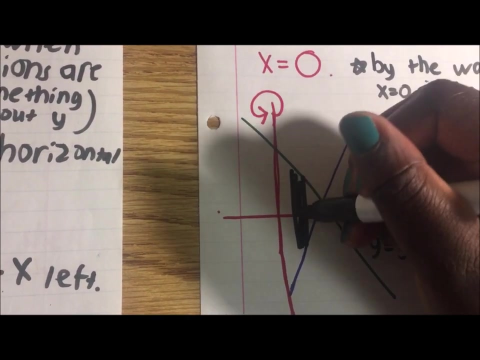 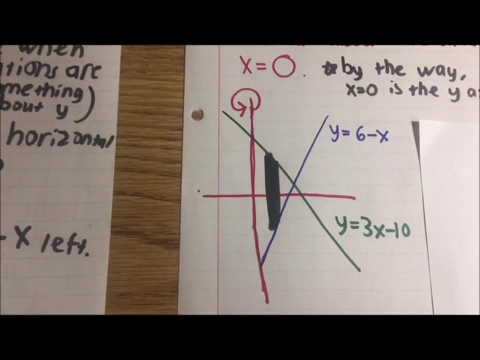 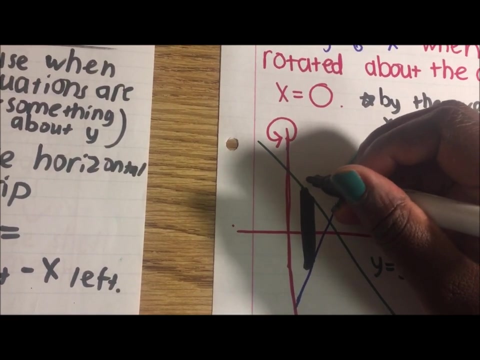 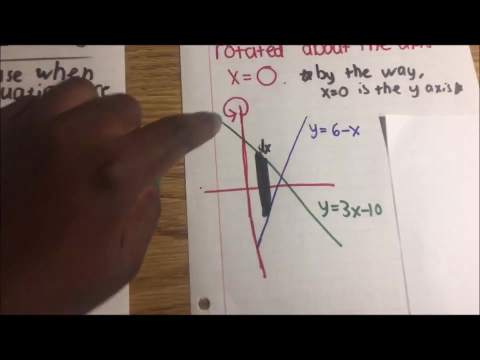 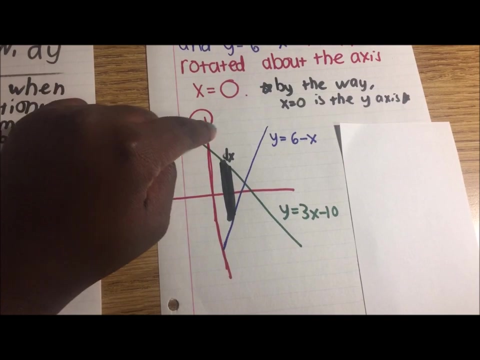 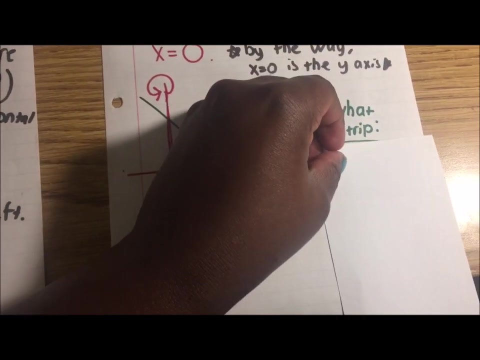 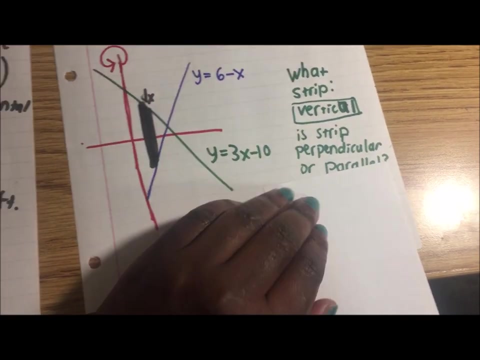 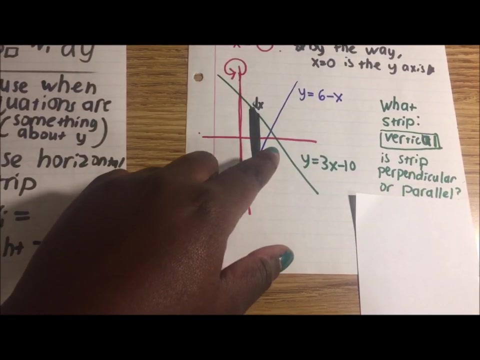 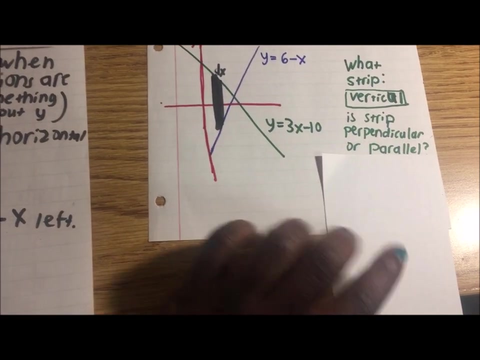 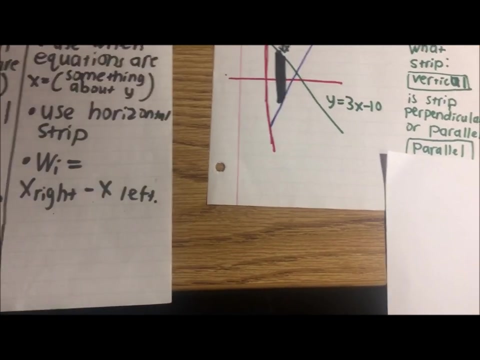 And then, so the equations are y equals 3x minus 10. y equals 6 minus x. So it's y equals something about x and y equals something about x. y equals something and here it's y equals something. So since it's y equals something about x, let's use another vertical strip let me draw that vertical strip this is a vertical strip oh yeah yeah that's the vertical strip the x-coordinate for this strip is X I and then this would be like DX here but the x-coordinate for the strip is X I but anyway um anyway here's the rotating axis the the rotated axis is X equals 0 which is really the y-axis so this is the rotating axis right here and then this is the strip so what strip we already said the strip was vertical is the strip perpendicular or is it parallel let's find out so this is the rotating axis this is the vertical strip and then this is the vertical strip so what this is the elastic loop and then we have aş forcing it parallel so understood so this is the axis receiving it背景 series Wa and this is the strip the strip is like this the rotating axis is like this therefore the strip is parallel to the rotating axis it's parallel so let's go back to our 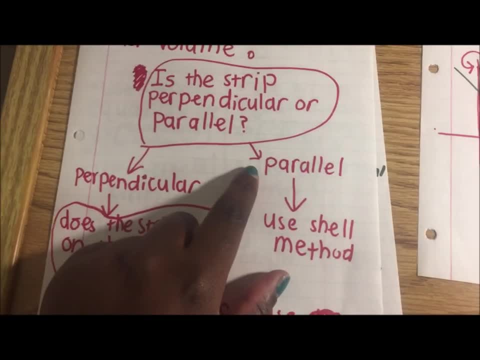 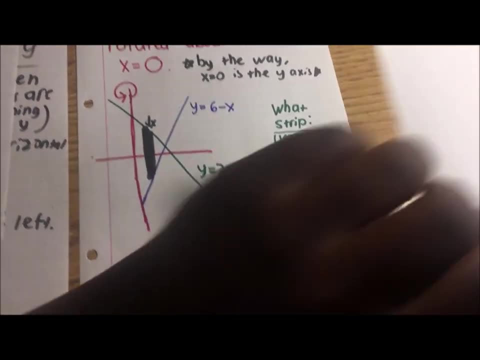 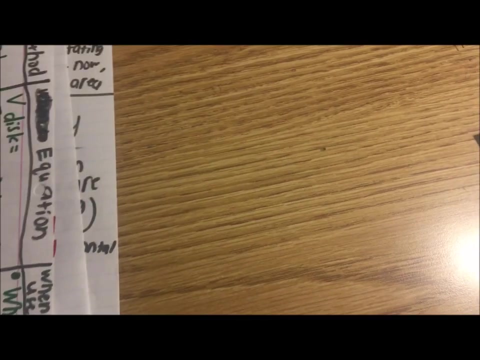 flow chart is the strip perpendicular or parallel to the rotating axis this strip is parallel to the rotating axis it's parallel the shell method because the strip is parallel to the rotating axis so basically um that's how